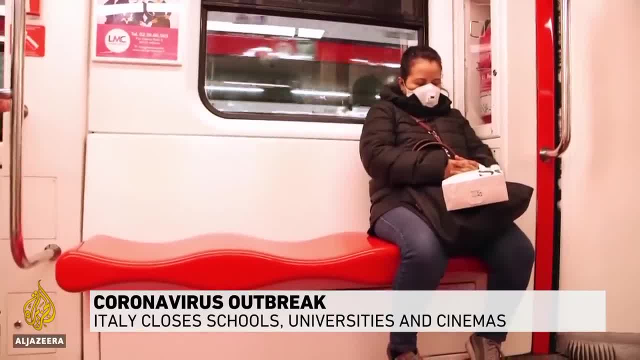 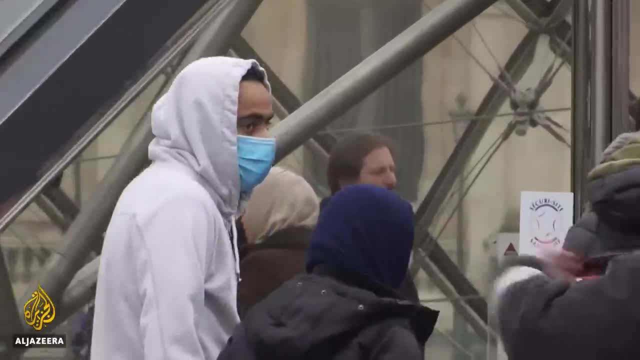 Contagion is spreading quickly across Europe and the world, and that means anxiety as much as the COVID-19 virus itself. Staff at the world's most famous museum, the Louvre in Paris, shut it down for three days this week, demanding better protection against the virus. 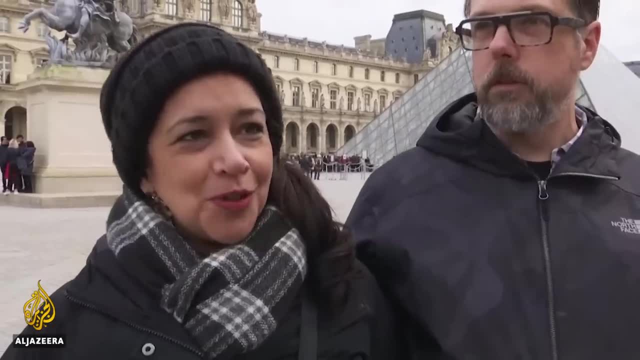 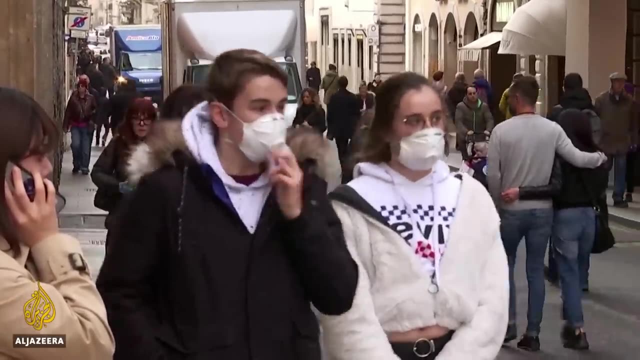 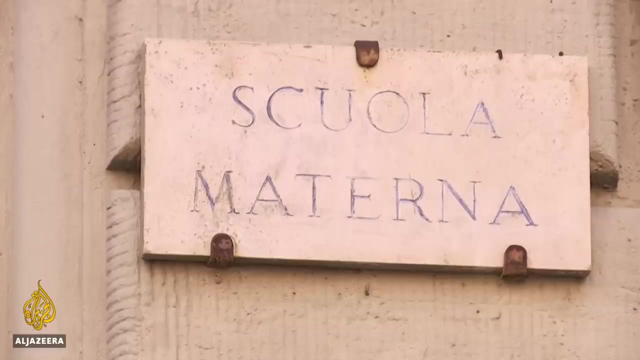 Tourists weren't amused. There isn't a place in the world that it's not going to get to, and you can't just shut down the world. You can, though, shut down parts of it. Battling Europe's most prolific outbreak so far, Italy will close all schools and universities until mid-March, in an effort to stem the tide of infections and a rising death toll. 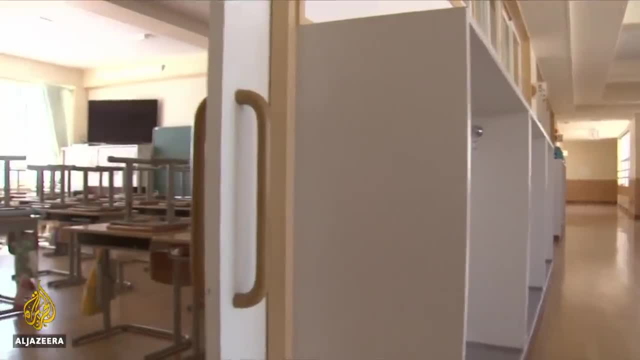 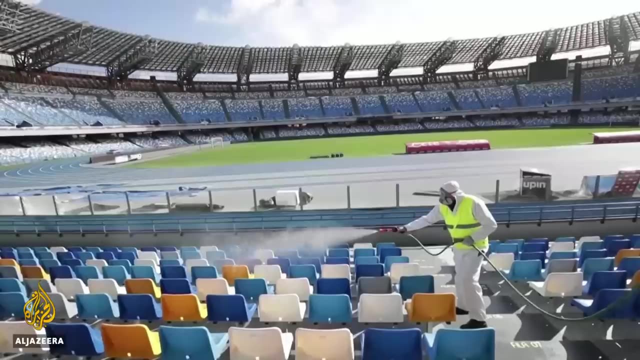 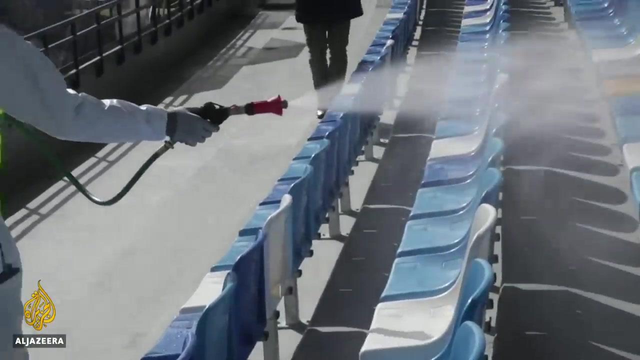 Japan did the same last week, and France has also ordered the closure of some schools, affecting an estimated 35,000 pupils. As dramatic for some Italy's decision to hold all sporting fixtures in empty stadiums, Spain has done so too. Life across the globe. 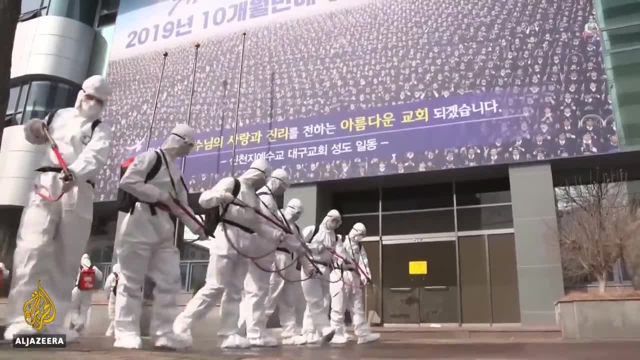 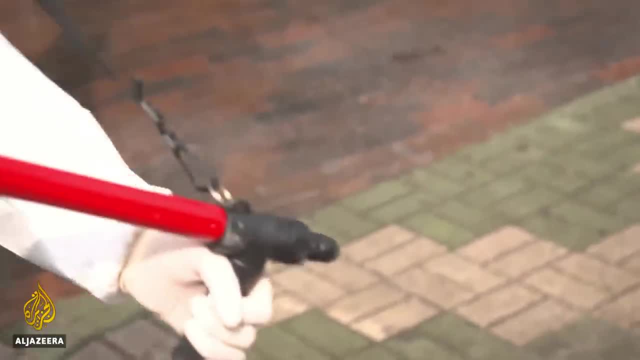 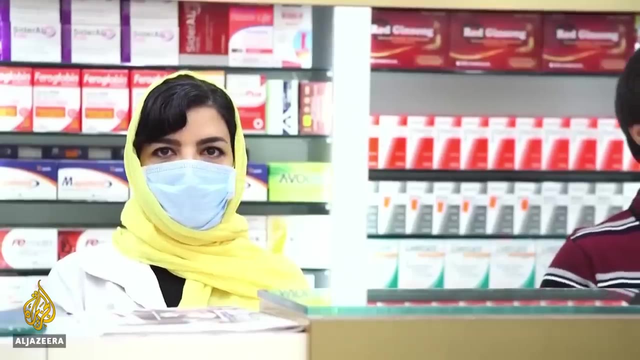 The world health organisation continues to stress the importance of containment in places with few infections, in the hope of delaying the spread of the disease and to give health systems time to prepare. There is no doubt that things will get worse, And if the WHO isn't yet prepared to declare a pandemic, Germany, it appears, is. 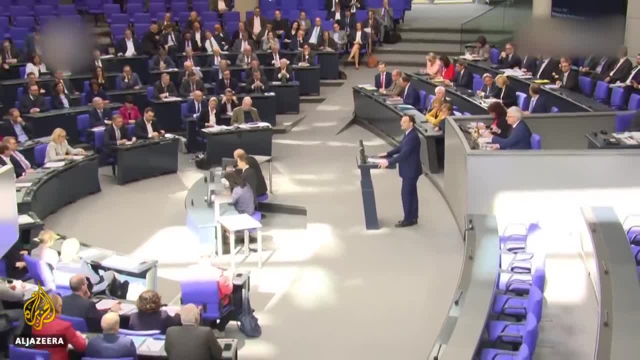 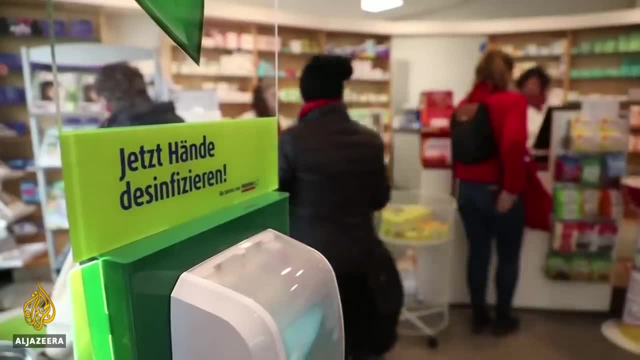 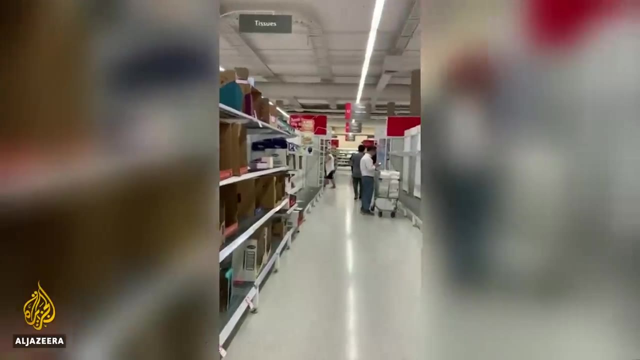 The coronavirus outbreak, said the health minister, has become a global pandemic. Amid a worldwide shortage of goggles, masks and gloves, Germany has banned the export of medical protective gear. They want it all to be available for use at home, And other shortages have provoked concern, this time in Australia over toilet paper. 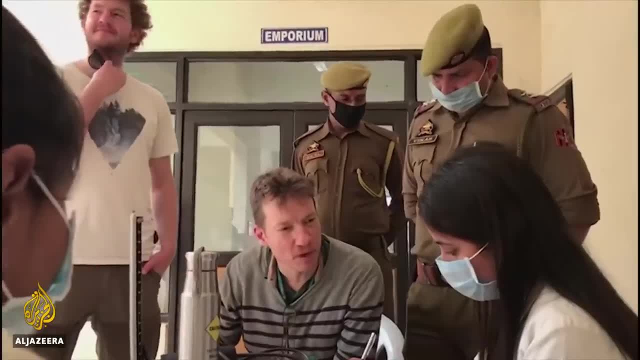 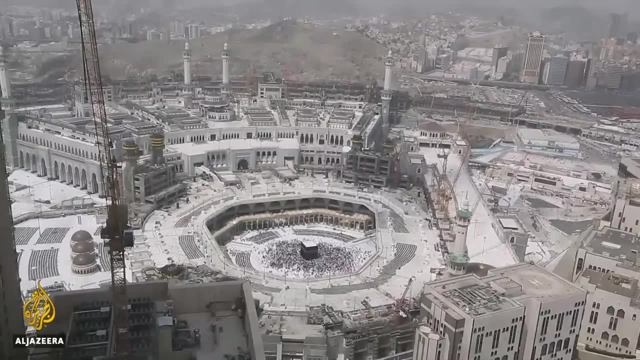 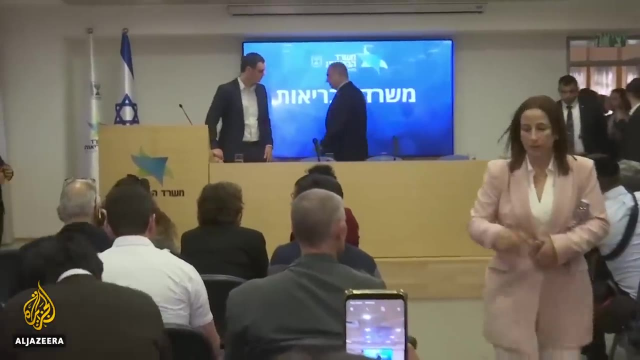 Some countries are taking matters steadily further. India has extended the screening of passengers to all those arriving on international flights. The authorities in Saudi Arabia have banned citizens and foreigners from taking the Umrah pilgrimage to Mecca. In Israel, Prime Minister Netanyahu suggested the common handshake be replaced by the Indian greeting namaste. 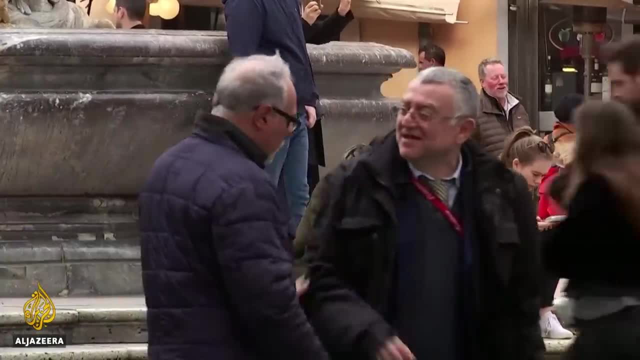 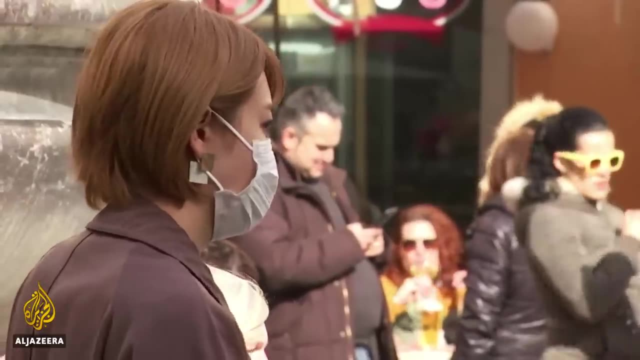 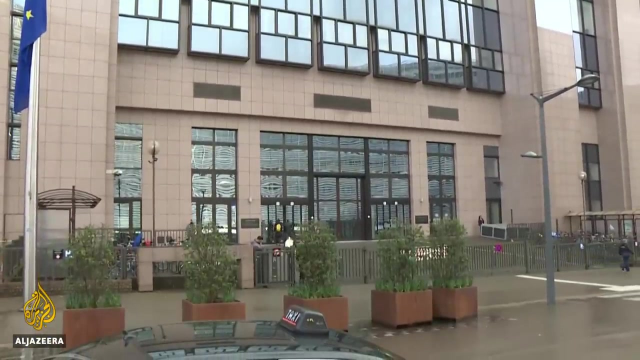 while Italians have been asked to stop kissing and hugging. With the Covid-19 virus reaching more and more countries each day, it is possible that no corner of the world will be spared. Even as European health ministers prepare to meet on Friday, one infection was registered inside the European Council building itself.